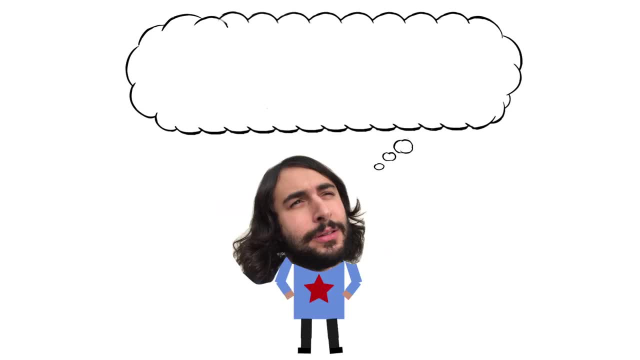 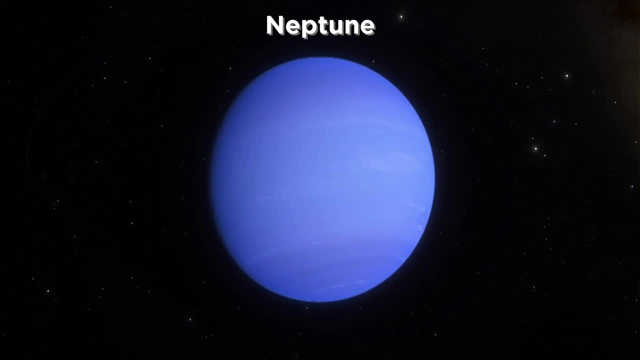 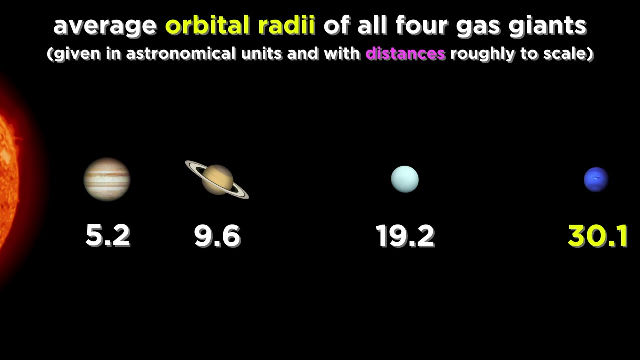 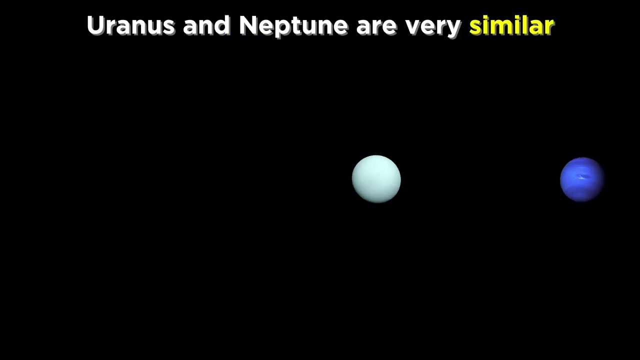 Professor Dave, here let's look at Neptune. Neptune is the last of the gas giants and the last of the planets in general. It is very far from the sun at about thirty astronomical units, about as far from Uranus as Uranus is from Saturn. 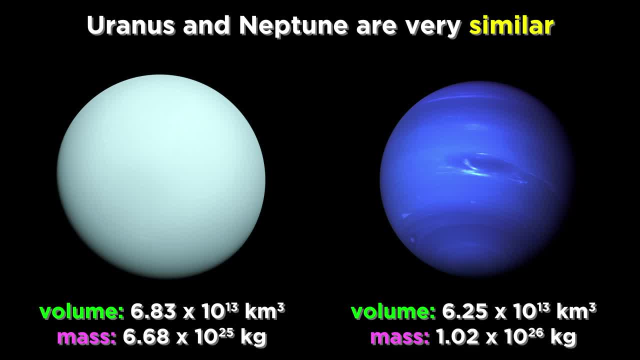 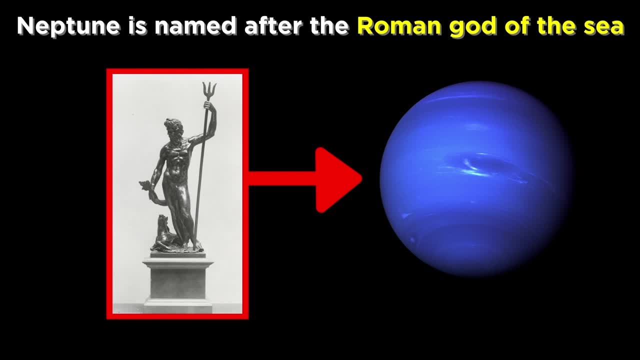 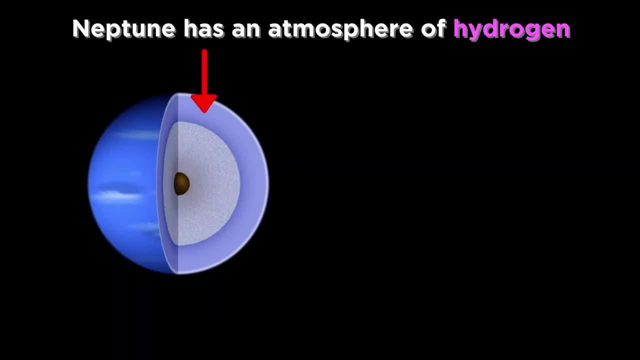 Neptune is quite similar to Uranus, nearly identical in size and mass. It is deep blue in color and is thus appropriately named after the Roman god of the sea. Also similarly to Uranus, Neptune has an atmosphere rich with hydrogen above a layer. 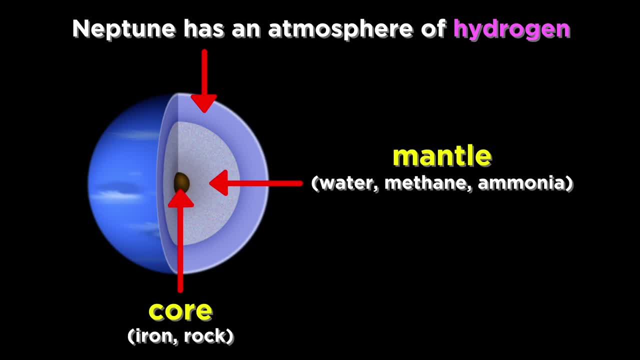 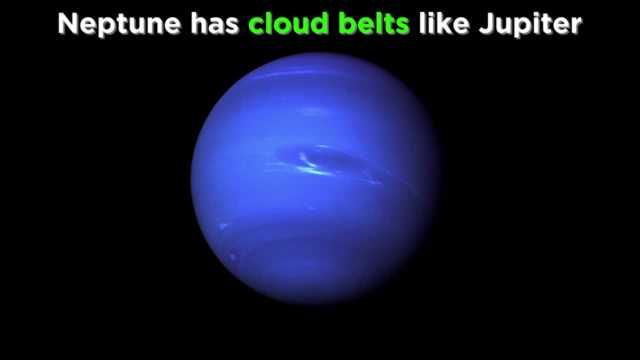 of water, methane and ammonia around a core of iron and rock. One difference between the planets is that Neptune has distinct cloud-like atmosphere, Cloud belts more closely resembling the surface of Jupiter. We have even seen a great dark spot, which is a huge atmospheric vortex similar to Jupiter's. 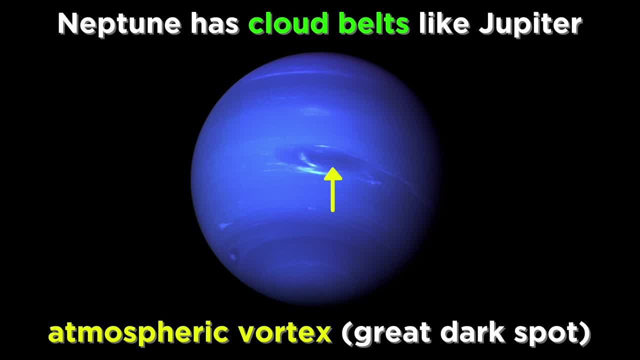 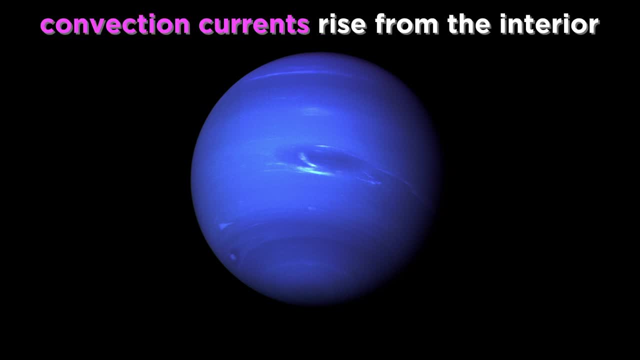 great red spot, although it is not a permanent feature, with similar spots forming and dissipating every few years. These features are due to convection currents generated by heat emanating from the interior of the planet, which in turn cause fast waves. 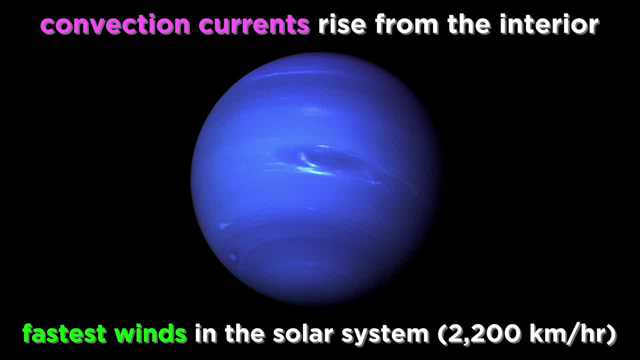 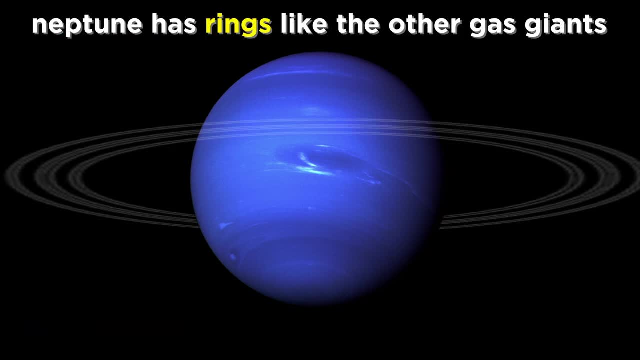 Neptune has the fastest winds, of up to 2200 kilometers per hour, the fastest winds recorded anywhere in the solar system. Neptune has rings, just like the other gas giants, although they are rather narrow, most likely comprised of debris from collisions between small moons or comets, as they contain. 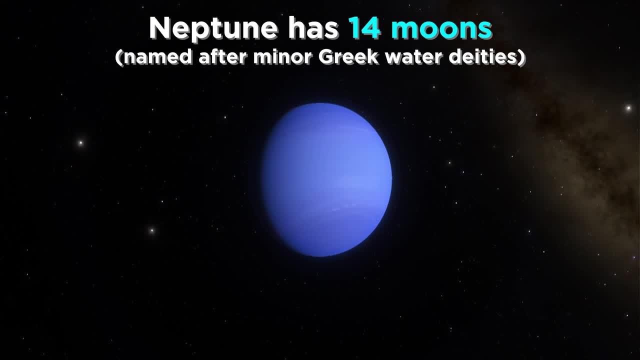 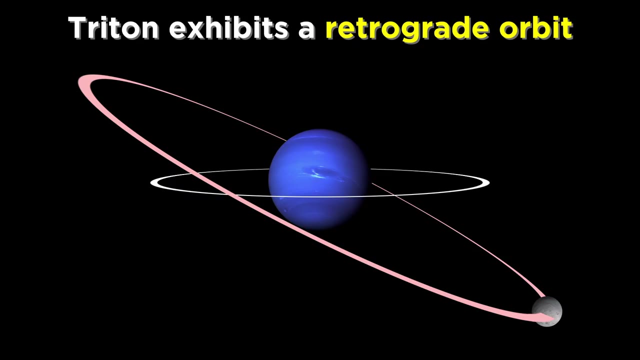 a lot of dust. Speaking of moons, the Neptunian system has fourteen of them, all named for minor water deities from Greek mythology. The largest of these by far is Triton, an icy world which strangely orbits Neptune in the direction opposite Neptune's rotation, which we call a retrograde orbit. 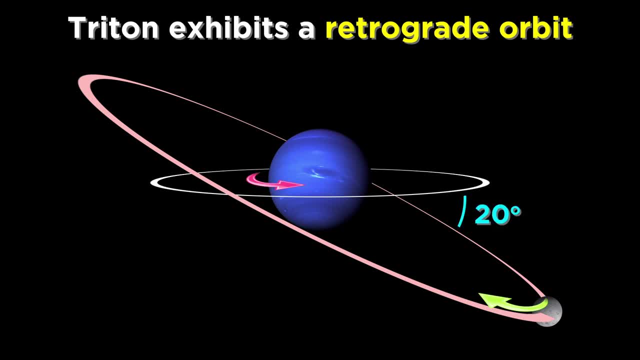 While Neptune spins one way, Triton goes the other, and with a significantly tilted orbit. This indicates that Triton was probably not formed from the same matter that became Neptune, but rather was captured by Neptune as a particle. This means that Triton was not formed from the same matter that became Neptune, but rather was captured by Neptune as a particle.